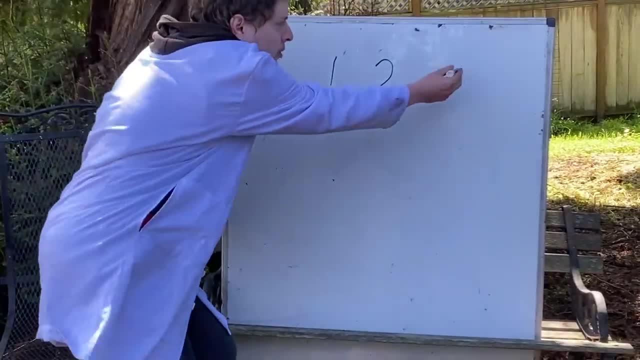 whether it's a multiple of two. Similarly with multiples of five, if the last digit's a multiple of five, the whole number is. So we're going to be looking at how to test whether something is a multiple of two or another one digit number, or even if their last digit is even. We only need to check. 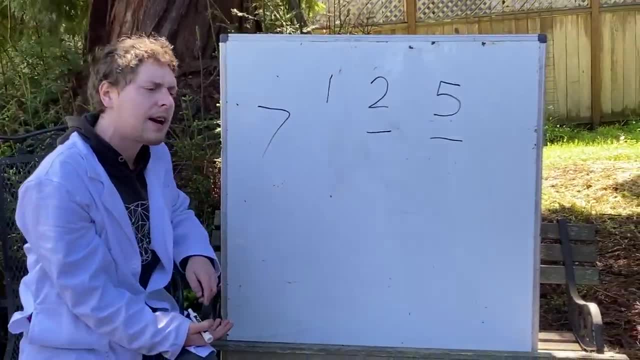 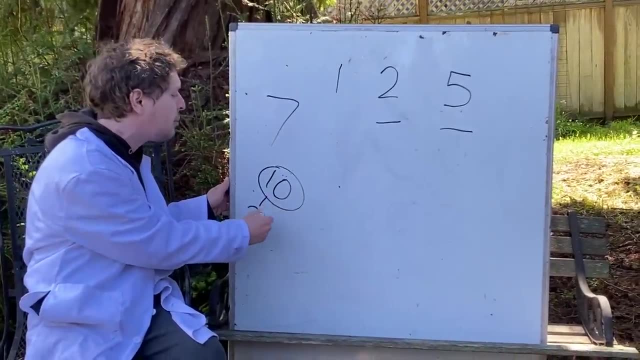 the last digit of a number to confirm whether it's a multiple of two or another one digit number. And if it's not, it's not. And twos and fives have that special trait because we count in a base ten system and tens prime factors are two and five. Now, if I add a number with more digits than one, 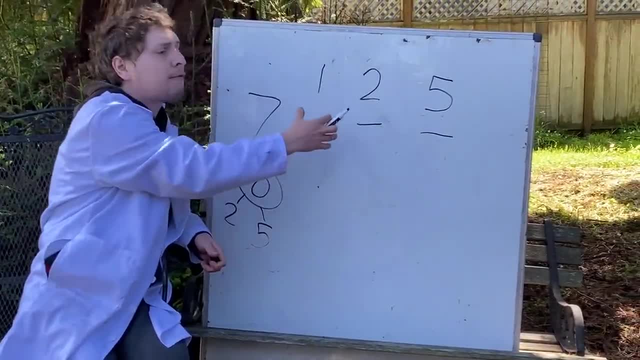 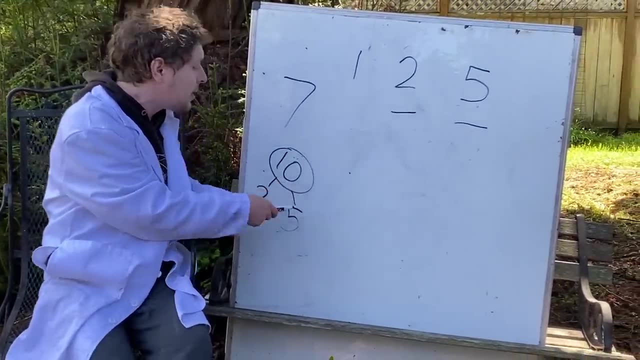 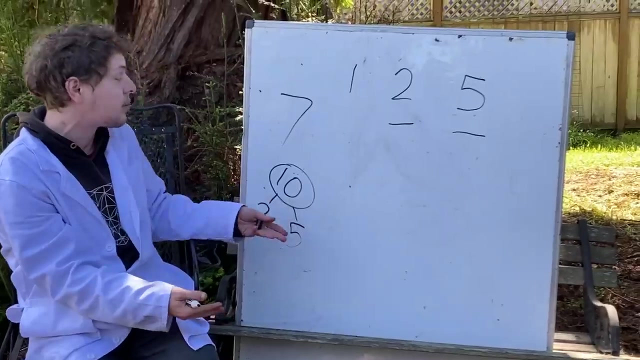 all of the digits to the left of the ones place are referring to an amount of tens, and an amount of tens, regardless of how many tens, is going to be divisible by two and five. So that portion of the number will certainly be referring to something divisible by either of those. We'd only need 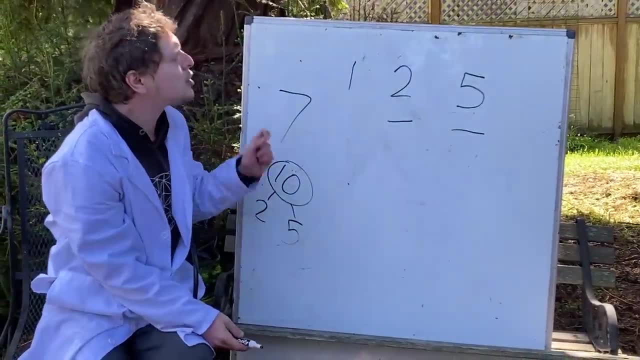 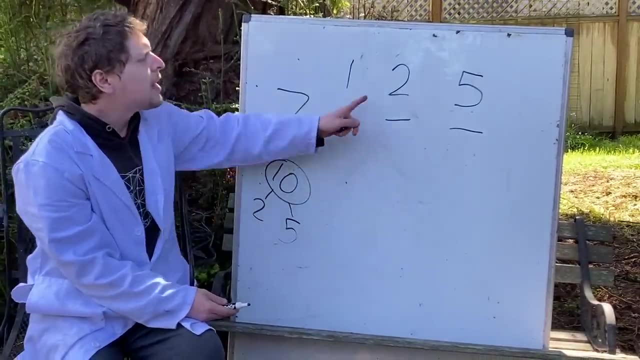 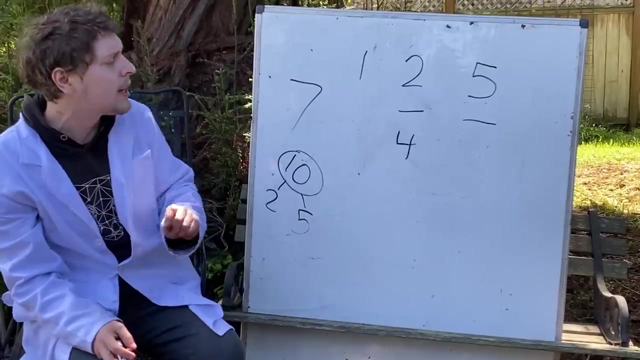 to check the remaining ones place And this power actually leaks forward to a degree to the powers of these numbers, For example, two to the second power is four and if I want to know if something is a multiple of four or if a number is divisible by four, in other words, I only need to check. 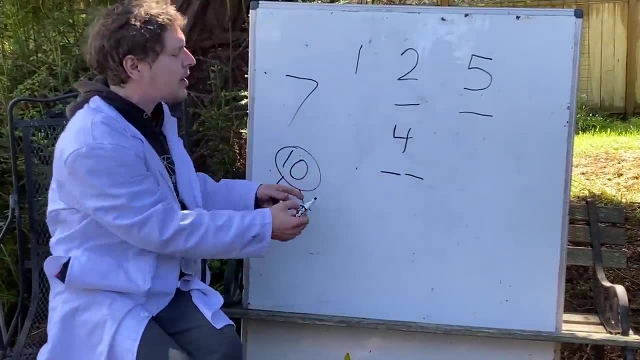 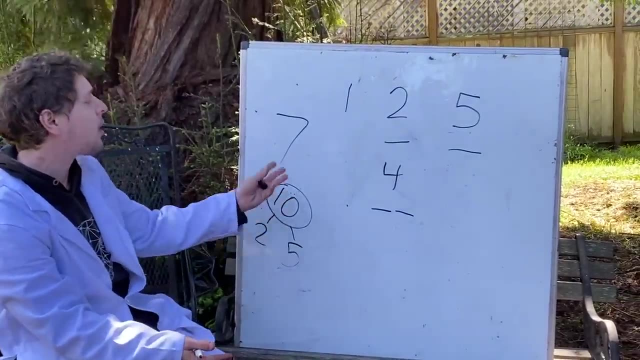 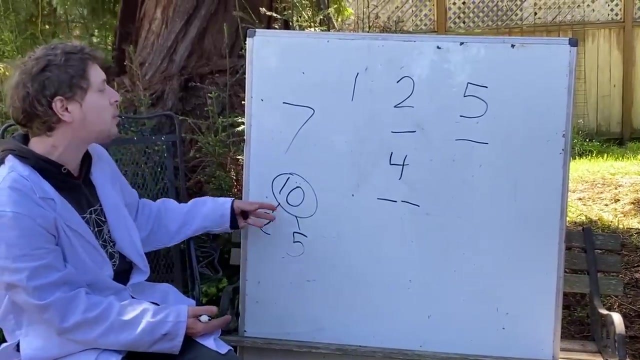 the last two digits, And that's because anything to the left of that in a number is referring to an amount of hundreds. in our base 10 system, 100 would be made up of a pair of twos multiplied by a pair of fives, And so then we're able to go to the next power and know that that portion of the 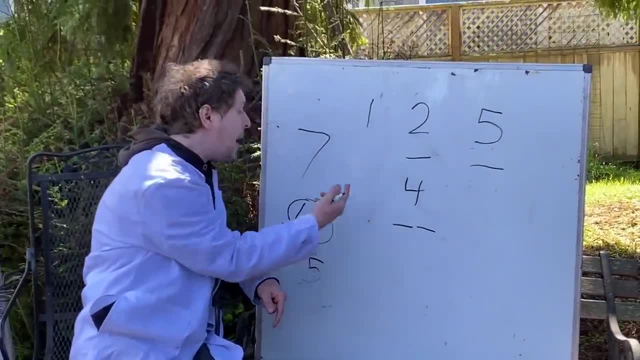 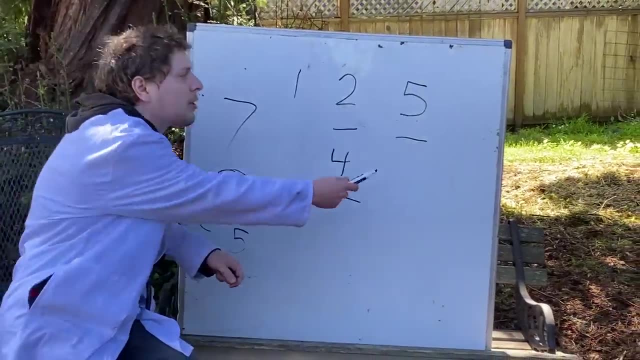 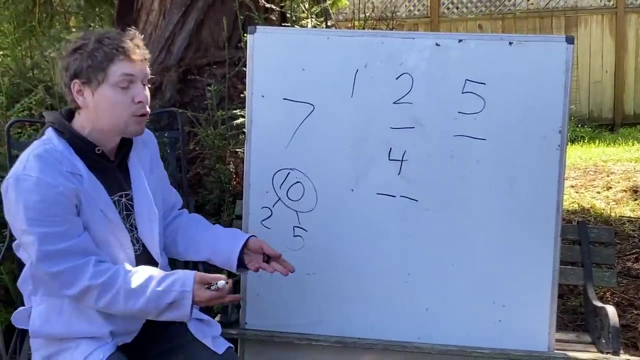 number would automatically be divisible by two squared And we'd only need to check the tens place and ones place. We could do a similar thing for 25 if I wasn't only focused on the one digit numbers where to check if something was a multiple of 25.. Due to that being five squared, we'd only 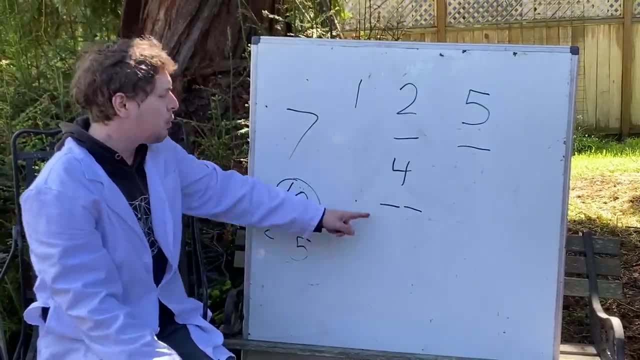 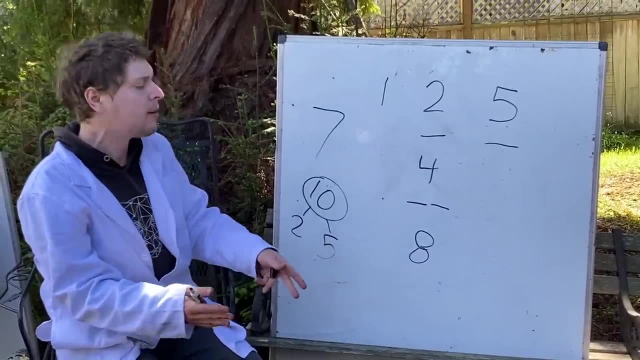 need to check the last two digits. Now, with eight, we can even take this one step further. Eight is two cubed, And to know if something's a multiple of eight, you only need to check the last three digits. If the last three digits 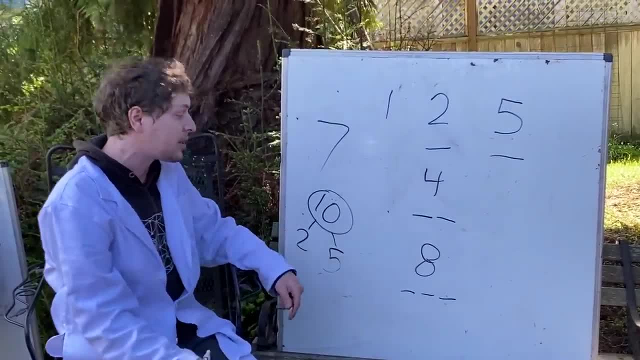 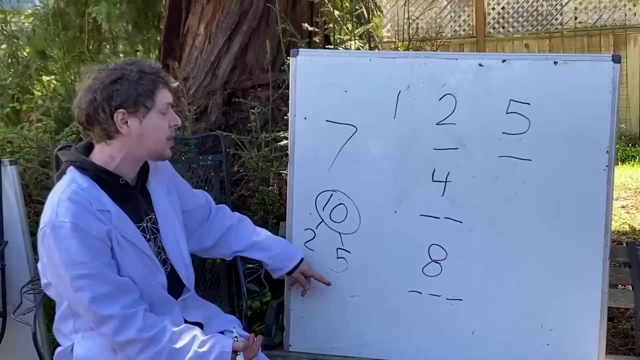 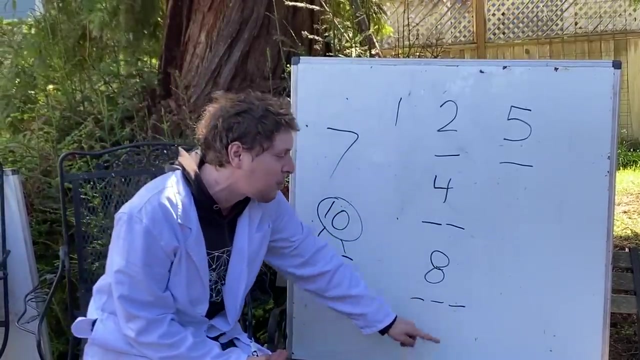 of a number are divisible by eight, the whole number is, for similar reasons, where the rest would refer to thousands. and thousands are divisible by two cubed times five cubed. Now, to check if something is divisible by one of these might get tricky at this point, because then how do you know? 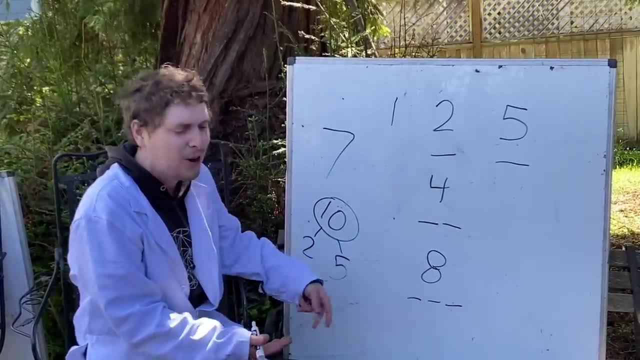 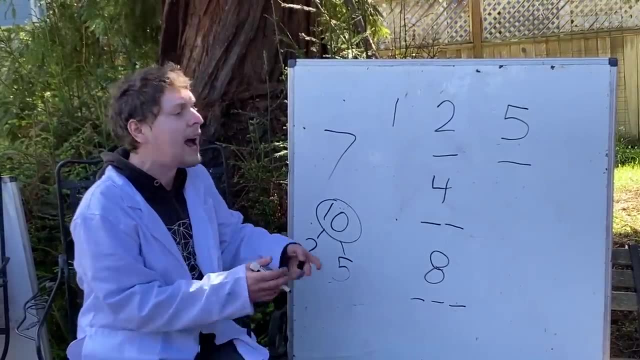 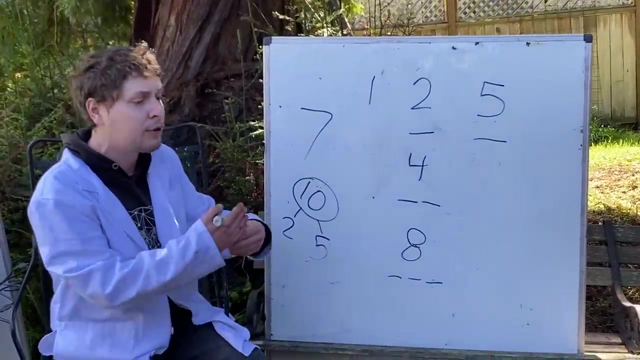 if the three digit number is divisible by eight, if it's a large enough three digit number. So the easiest way to go about that would be to split the number in half. If you can split something in half once and it is still a whole number, then it's even. but even already had an easy trick. So 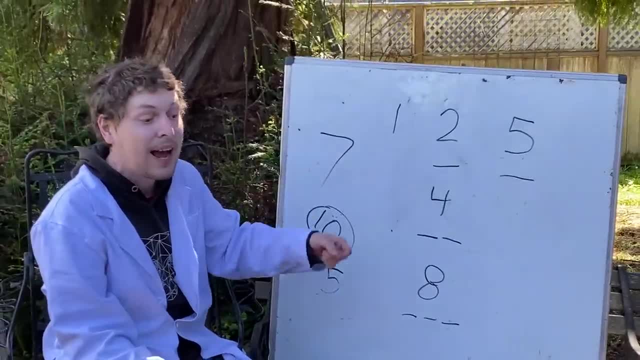 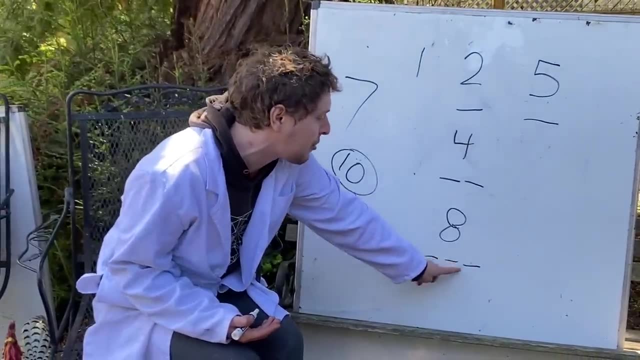 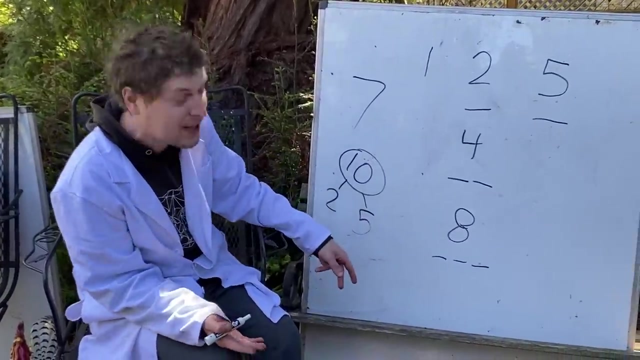 if you split it in half again, and you've now cut the number in half twice and you still have a whole number, the number was divisible by four, And here we could split the three digit ending in half, in half, in half, And if after all that three times we halved it, we still had a whole. 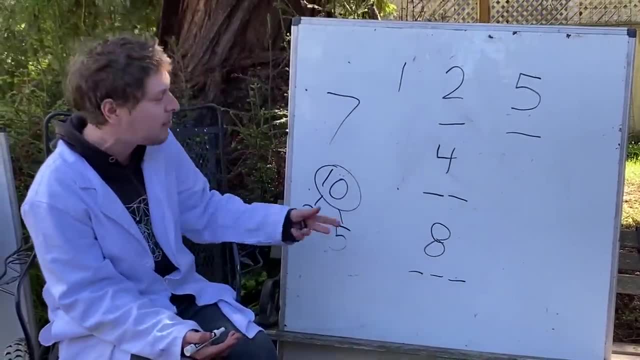 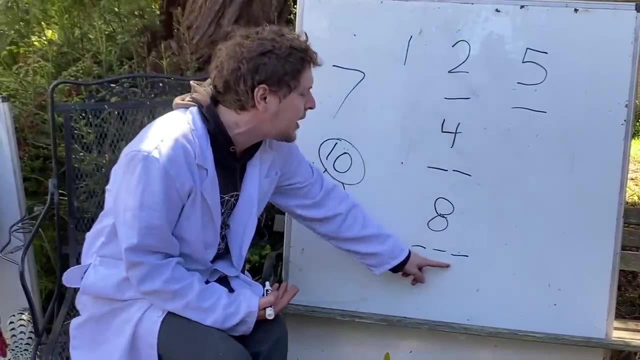 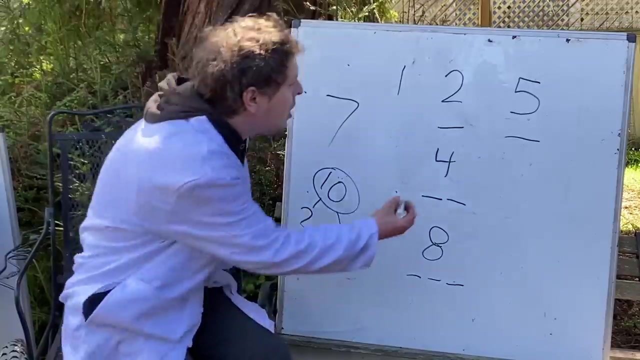 number, that would be a multiple of eight, and so would the whole thing. So not as easy as testing a multiple of two, but still inheriting this sort of easy-ish trait by being a power of two. Now, if I want to fill in the missing numbers, here we have three, six and nine. 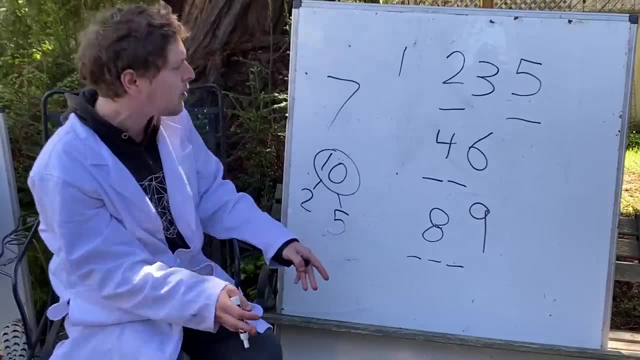 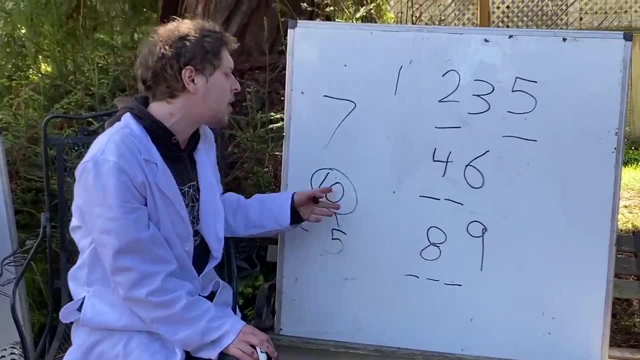 Now we might think that these are going to be harder to work with because these don't have these pure factors of 10.. Six has one factor in common with 10, but three is not one factor in common with 10, so it's even harder to work with that. So this way, 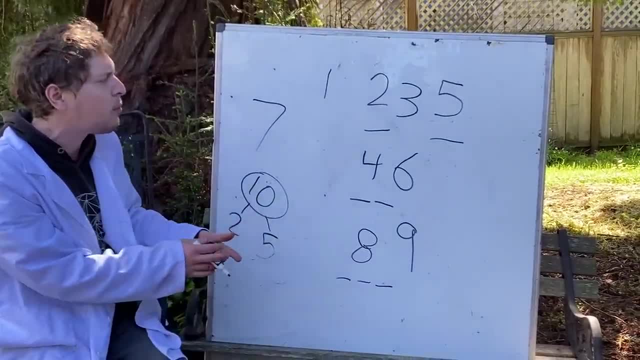 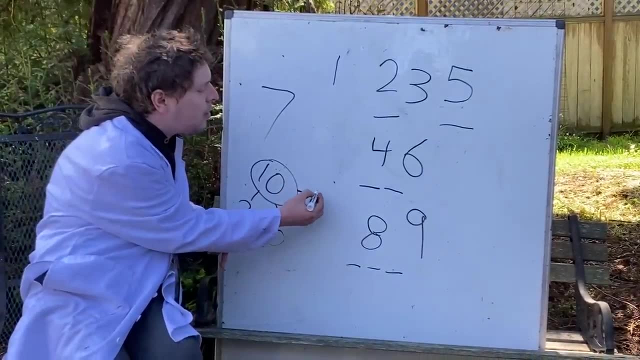 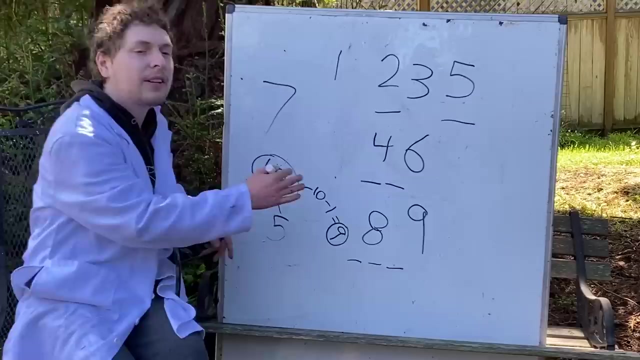 3 and 9 don't even have any factors in common apart from 1.. However, 3 and 9 have factors in common with 10 minus 1, which is 9.. The number that, in our base, has these special divisibility properties. 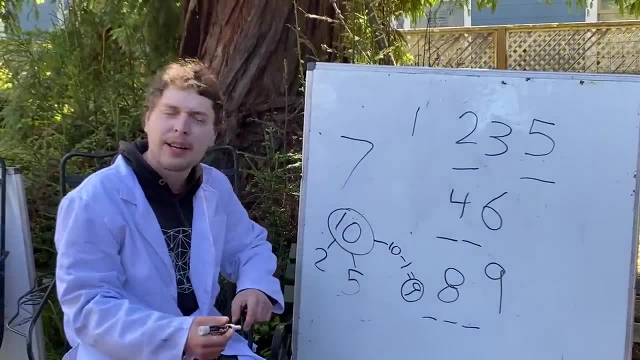 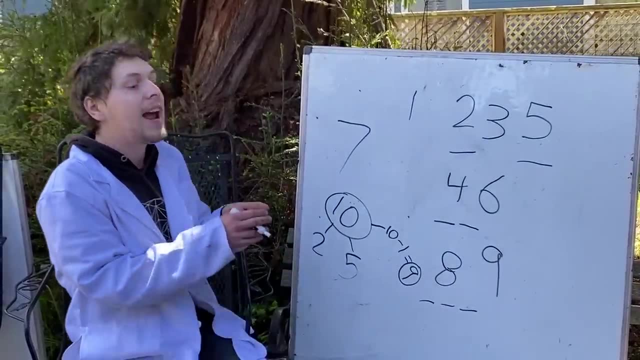 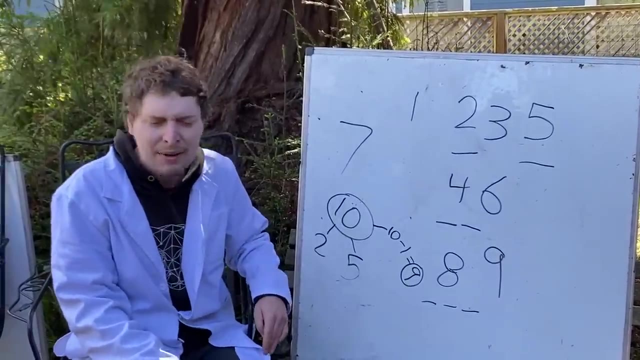 that the number 1 less than any given base would have, And that means that for multiples of 9, if I add up all the digits in a number and that result is divisible by 9, then so is the whole number. It's a different technique than checking the last amount of digits. 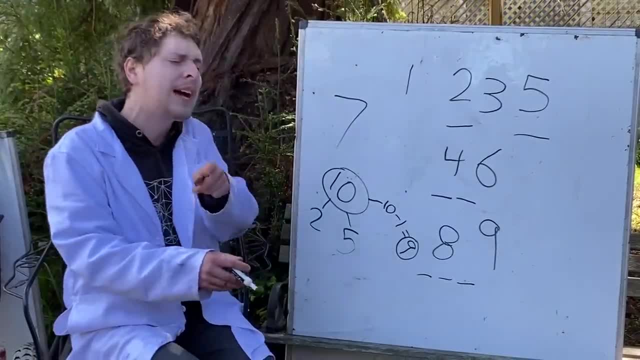 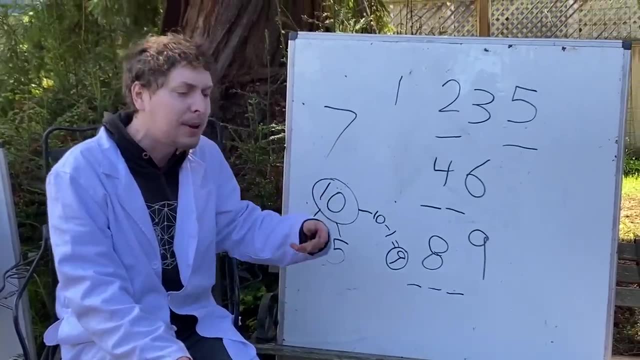 You add all the digits, And if you don't know if that's a multiple of 9 yet, you can add them again. If you repeatedly add the digits, taking the digital sum until you get the number 9, you can add them again. 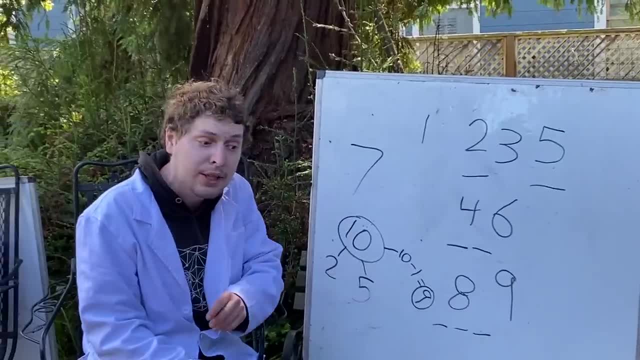 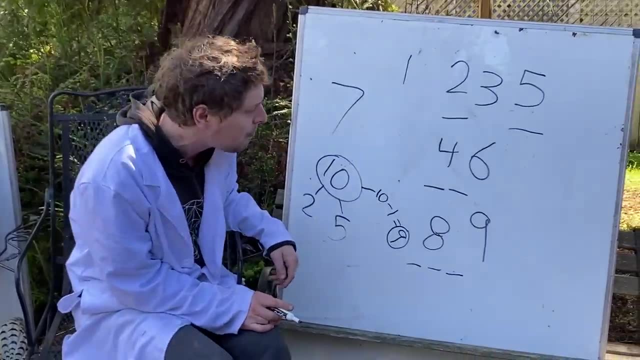 Until you're at the digital root, which is when you're down to one digit, multiples of 9 will always end up on the number 9 and no other types of number will. So here we can do a trick that I'll write with a little plus. 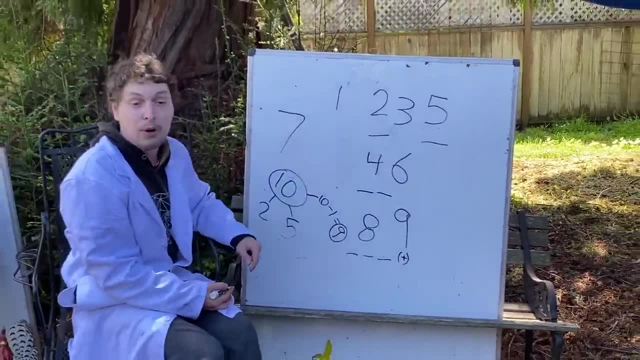 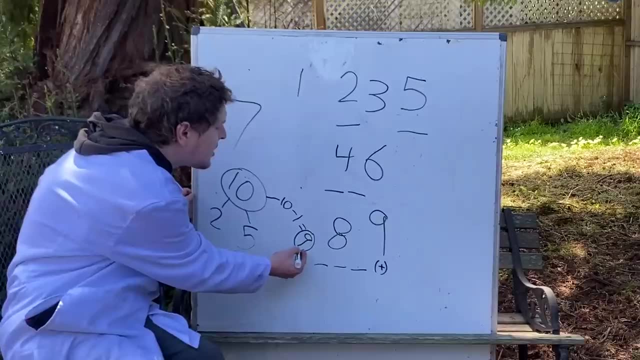 meaning if you add the digits, you can know whether it's a multiple of 9 by repeatedly adding them downward. But we get that additional trait here as well, because 9 is made up of 3 squared, It's a 3 times another 3.. 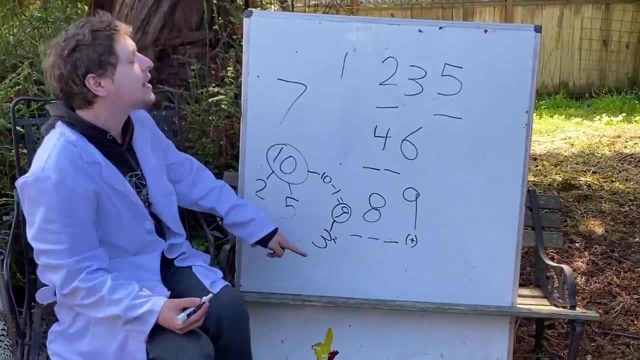 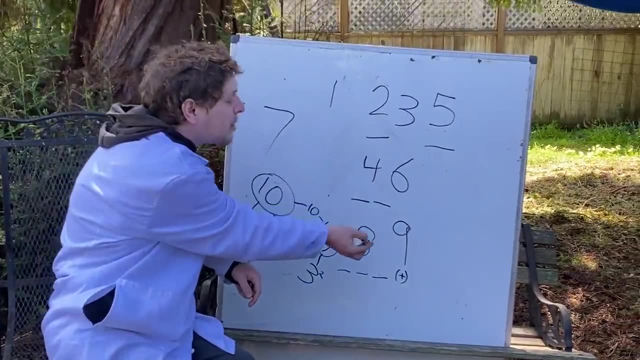 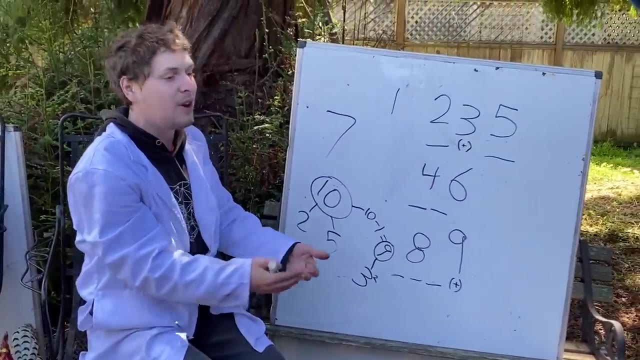 But in the prime factoring of 9,, 3 inherits this trait, where multiples of 3- that I call threven numbers- have the similar trait of: if you add their digits you'll get another threven number, And if you add the digits of a non-threven number, 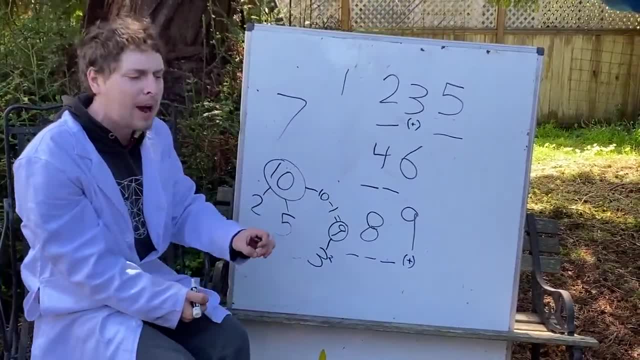 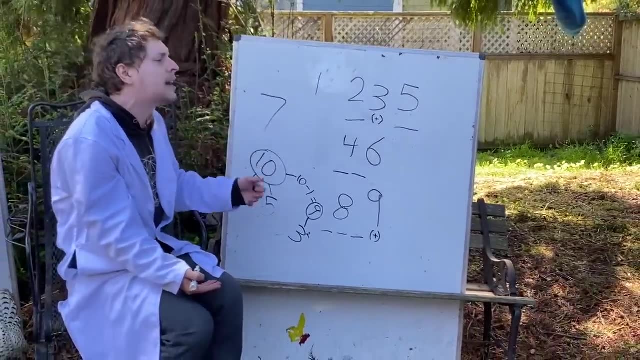 your result won't be threven. And you can also continue that process where, if you keep adding the digits until you're down to the single digit digital root, if, and only if- it's a threven digital root one of these, it's a multiple of 3.. 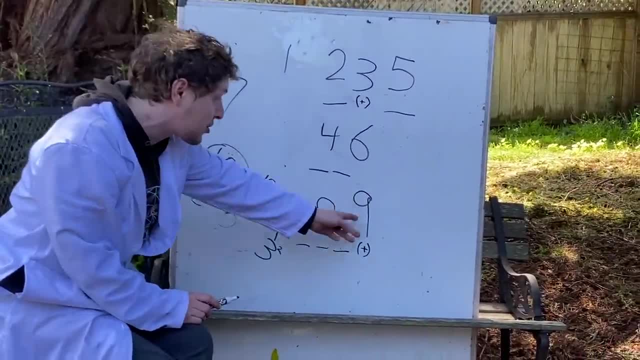 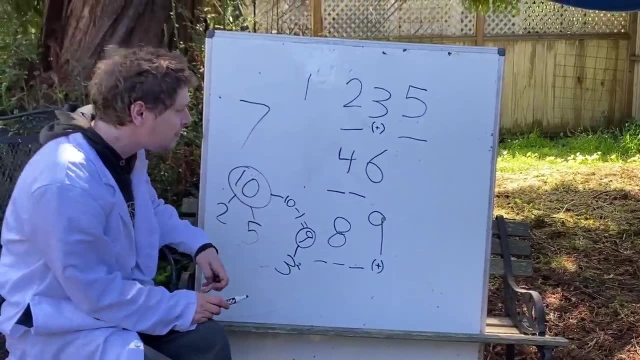 And if it's the 9,, then it's also the multiple of that second 3 in there and is divisible by 9,, what I call doubly threven. Now, as for 6,, we can just do a combination of 3's trick and 2's trick. 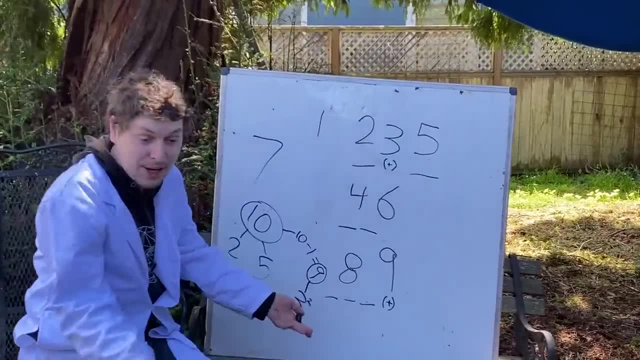 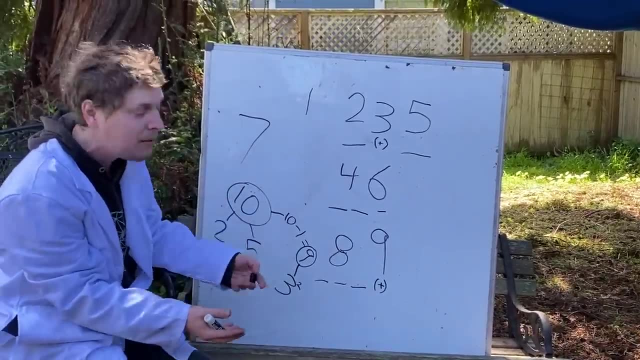 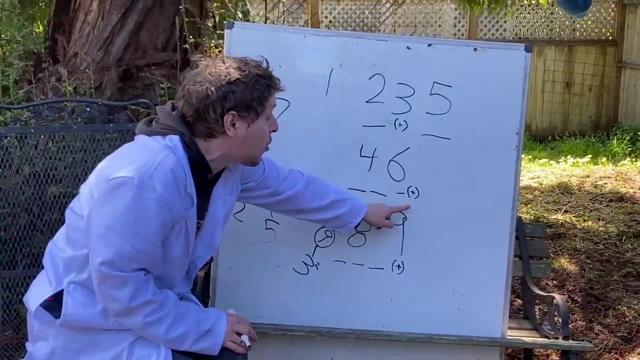 because 6's prime factorization is 2 times 3.. Okay, do is check if the last digit, just the last single one's place digit, is even and if the digits add to something threven, and if both of those rules hold and are passed, then the number is a multiple. 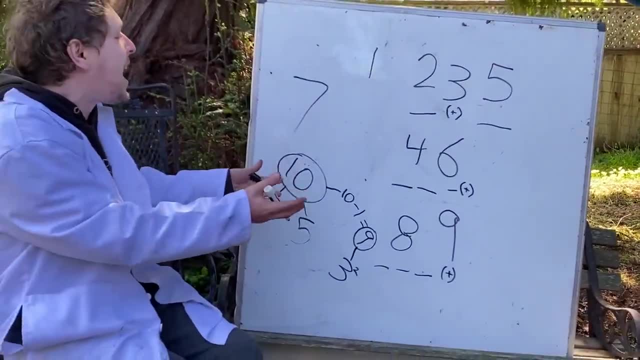 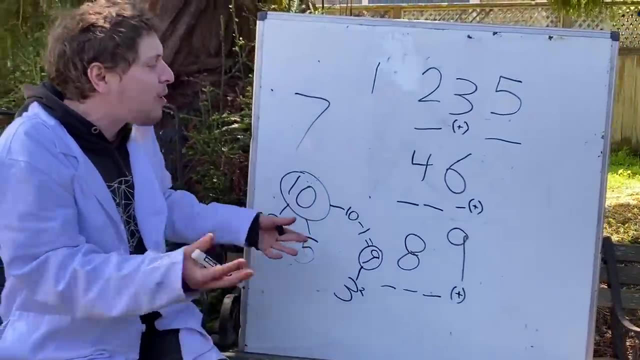 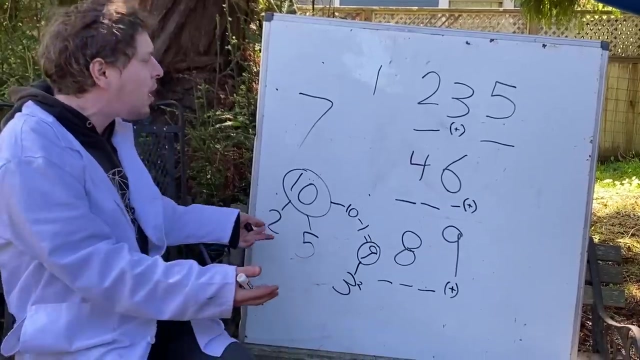 of six. now this leaves out seven. if you look up divisibility tricks for seven, there are a few options, but they're all really complicated and practically unuseful. at that point you might as well find a calculator. one of the divisibility tricks for seven, for example, is to take all the 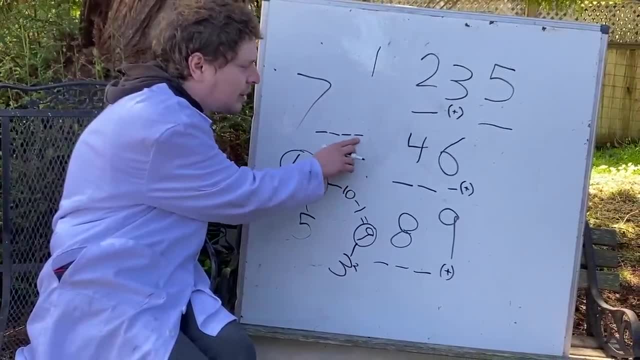 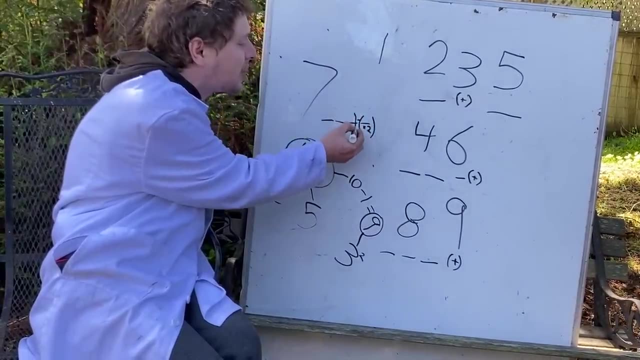 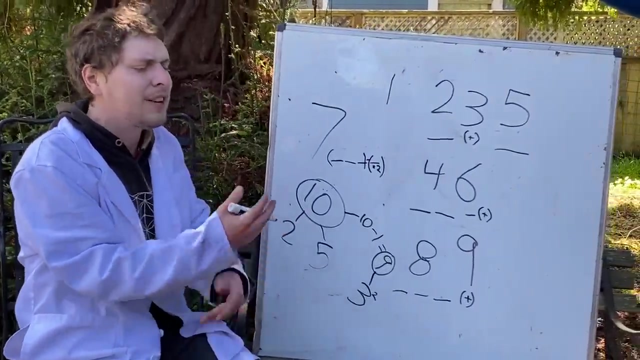 digits in a number. take just the last digit, the ones place, double it. find the difference between that doubled last digit and the remaining number and see if the difference is divisible by seven and then iterate that process if you don't know, and the other divisibility tricks for seven. 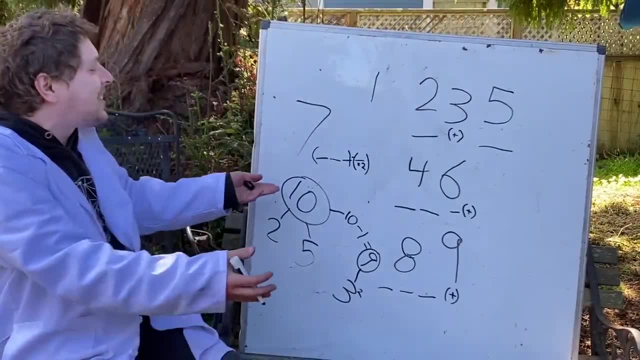 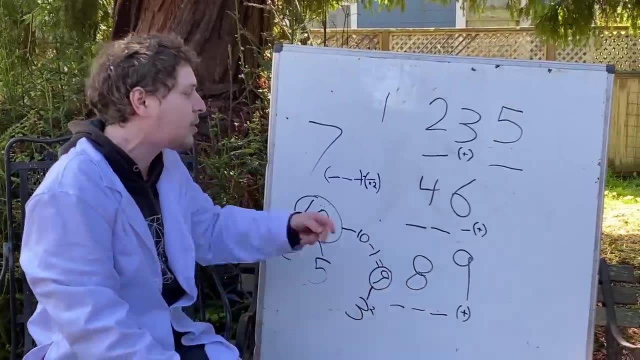 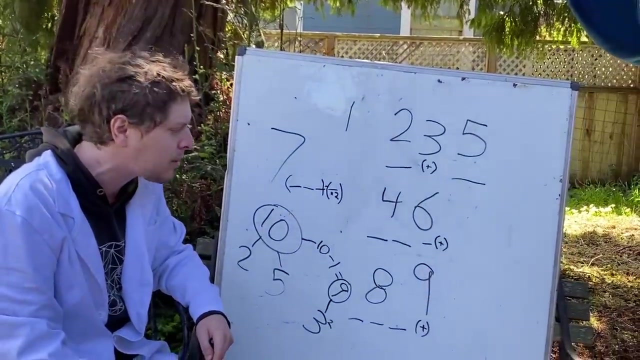 are similarly complicated. so why is it that seven didn't get any cool simple superpowers when all of these other single digit whole numbers did well? this relates to the fact that seven has a weird trait out of the single digit numbers. if we count all the numbers from one through ten, including ten, 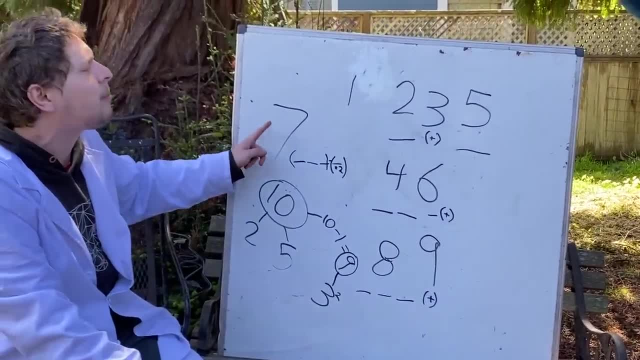 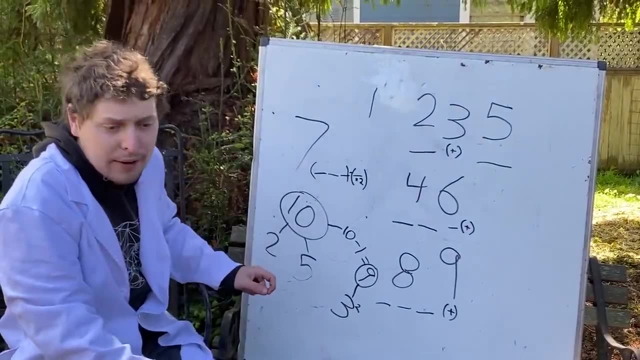 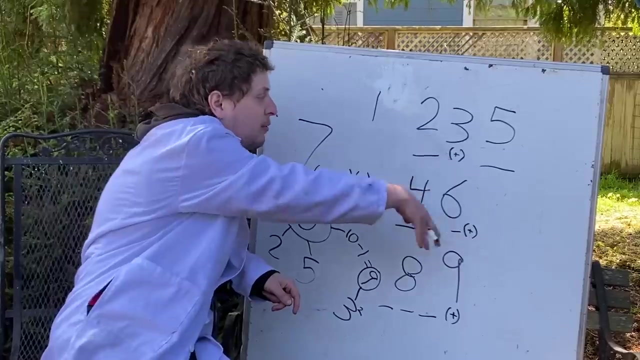 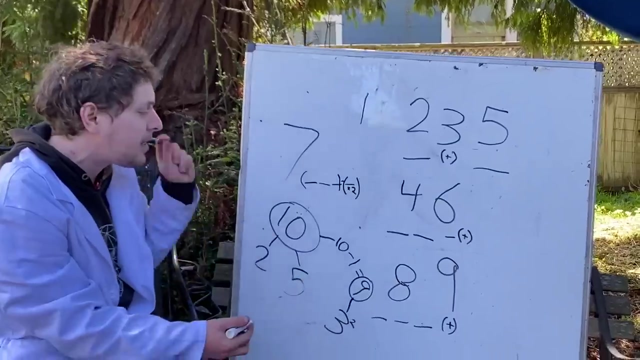 the base number, seven is the only number, apart from one, that has no factors larger than one, not only in common with any of these. all of these have some factor in common with one, of another one or with ten, but seven not only doesn't share with those, but specifically. 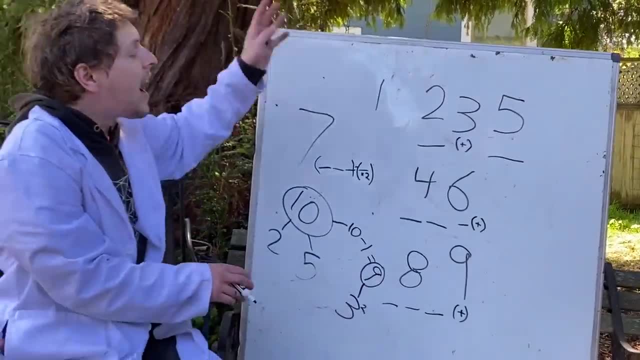 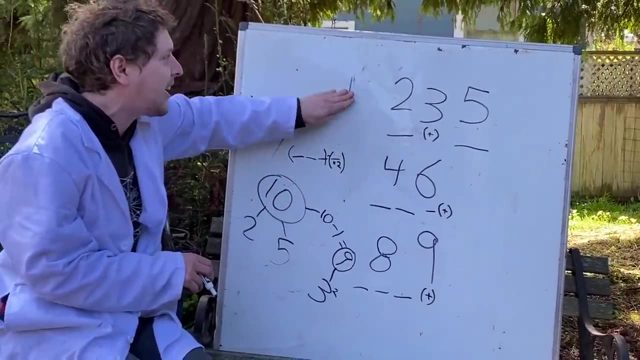 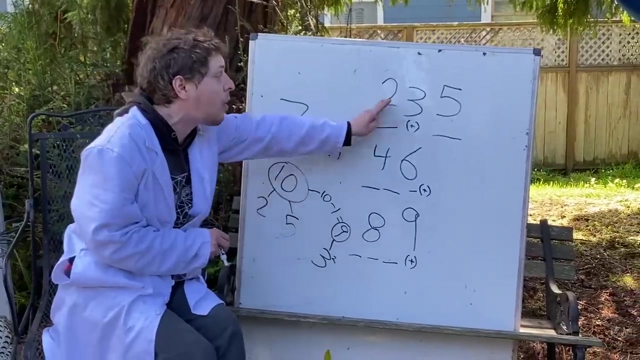 doesn't share them with ten and nine, whereas every single one of these. we do see some variation on the other side, as the number will be divided into three actions. we see this: one has varieties and one has variety, and the third one has complex. however, another factor that's given to us is figure of one of these, all of these larger than 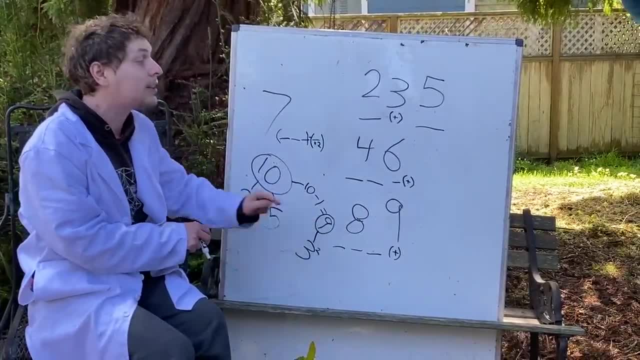 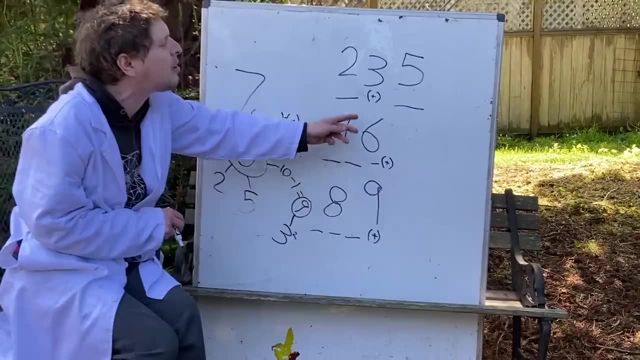 one which got a free pass where everything was divisible by it. all of these other ones have some factor larger than one in common with either 10 or one less than 10.. these ones have a 2 in common. these ones have a 3 in common. that also, oh, no, wait, they don't. uh, well, yeah. so they have a 3 in common with the 9 yep database, and 6 has a 3 in common with the 9, with 100, but they have a 3 in common with the 10.. 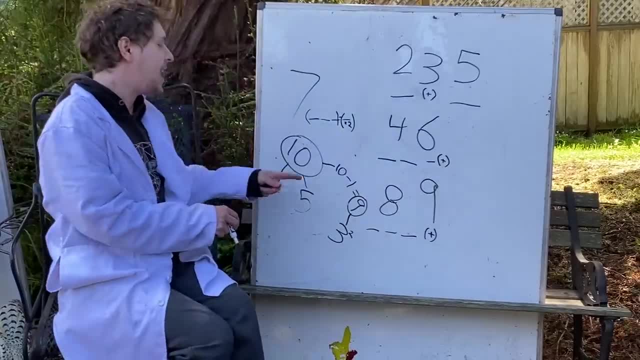 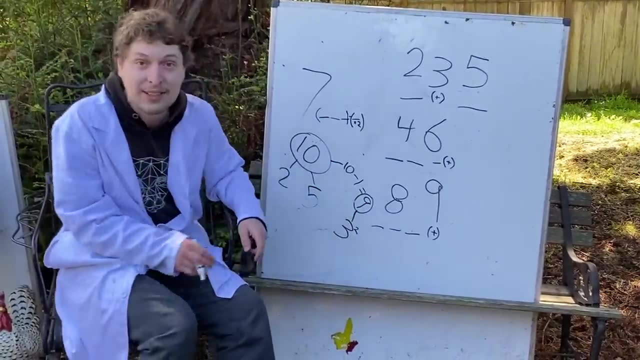 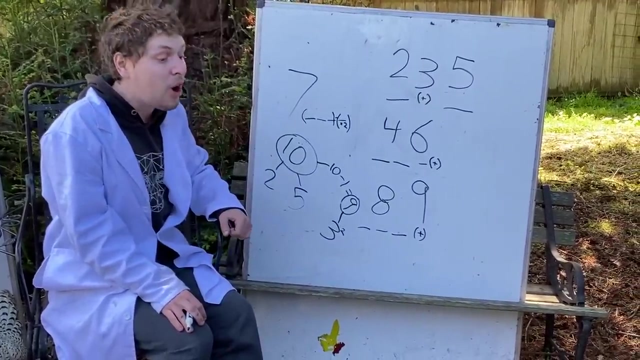 and a two in common with the ten. Five has the five in common with the ten. Seven has nothing in common with the base number or one less than the base number, And it turns out that that makes it our outlier, where it's much harder to test if a number is divisible by it, And that's one of the